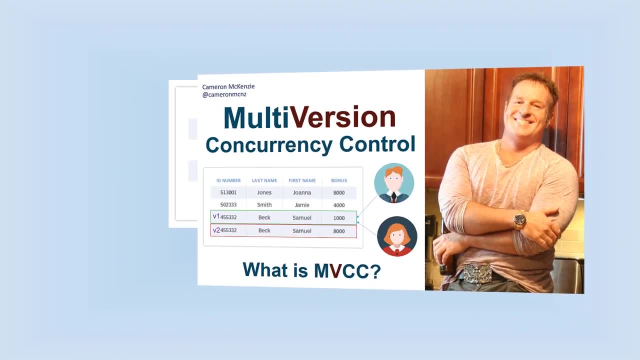 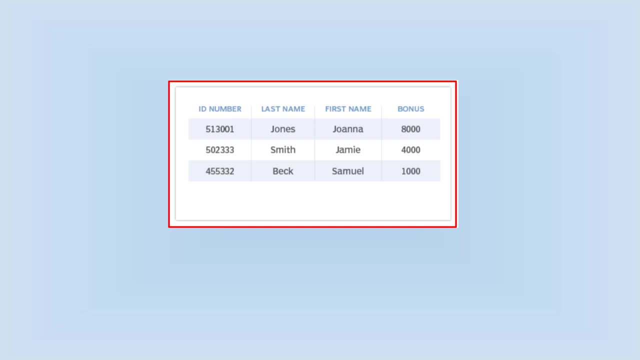 hey, i'm cameron mckenzie. i'm the editor-in-chief at theserversidecom and i want to quickly show you how multi-version concurrency control works. now, as you can see here, i've got a database table and there's something wrong with it, and what's wrong with it is the fact that samuel beckett. 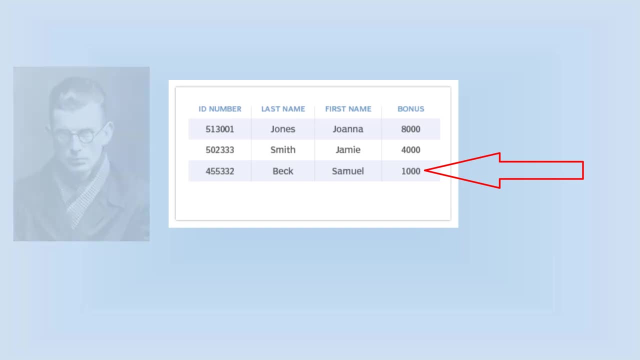 is only getting a thousand dollar bonus there and that's got the attention of the office. certainly nancy's come in to do a query of that database to see if that's true and nick's come in to do a query of that database to see if that's true as well. and the nice thing about a read operation: 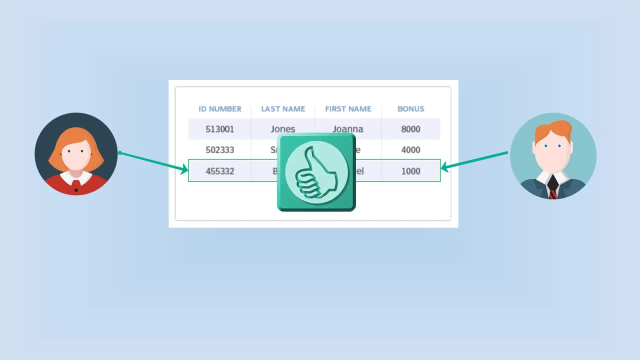 it's a safe operation, so you don't usually lock a row when multiple people are just going to be reading it. so nick can come in, nancy can come in and all sorts of people can come in and read that record and there's no locks. but you know, we've got the attention of mike and mike has decided to. 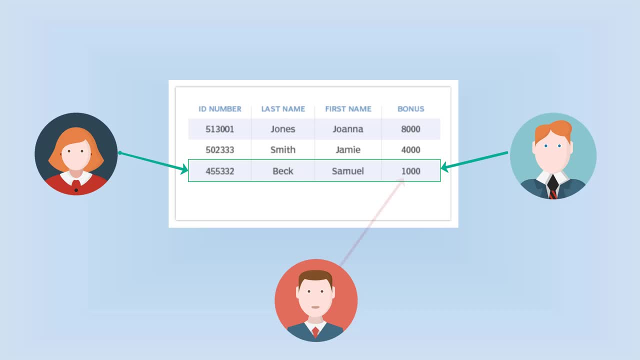 write this wrong. and what he wants to do is he want to update that bonus to 8000. so what does he do? he doesn't update. but here's the problem with updates: in traditional databases they lock the row, they lock maybe even the table, and that's not a good thing, because at that point, 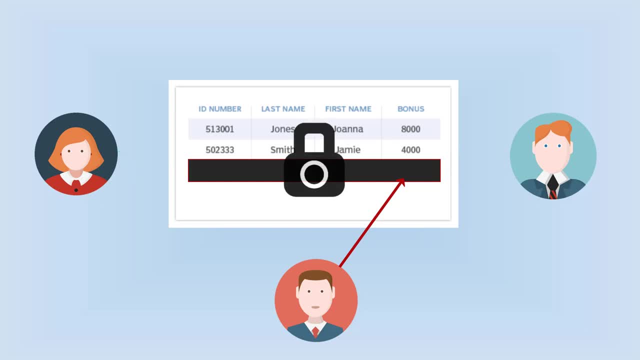 anybody who wants to do a read operation is locked out. that can cause, well obviously, concurrency problems because people that want to read the record can't gain access to it. potentially could lead to deadlocks, it could lead to lost transactions, failed transactions and it can just slow your website down. 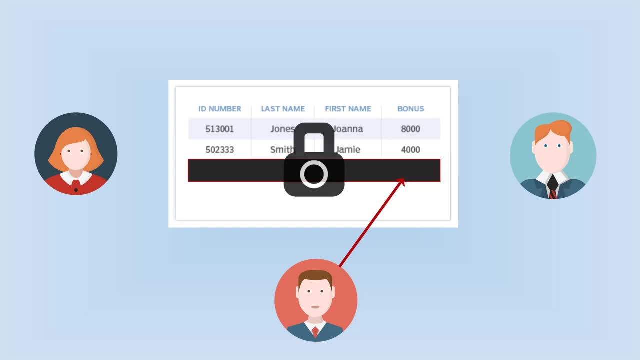 i mean, it's a horrible, horrible situation, but that's what we've done for the last 500 years of databases. we locked the record, we locked the row, we update it. you can see that mike's done a good job. now the bonus for samuel is 8 000. and well, the next time nancy or nick goes in to read: 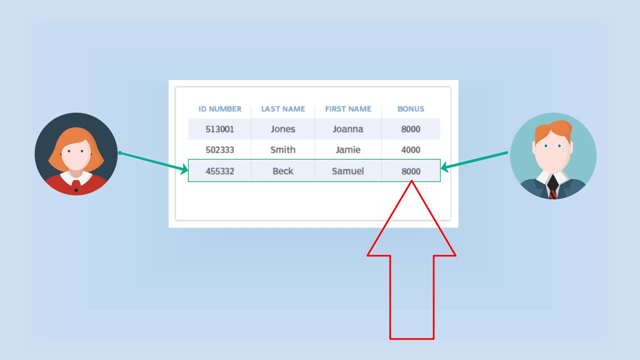 that well, they'll read the updated data. but there was that contention problem, that concurrency problem, a potential deadlock problem that we want to get rid of, and this is where multi-version concurrency control comes in. with multi-version concurrency control, anytime somebody reads a record, they also query the highest version. 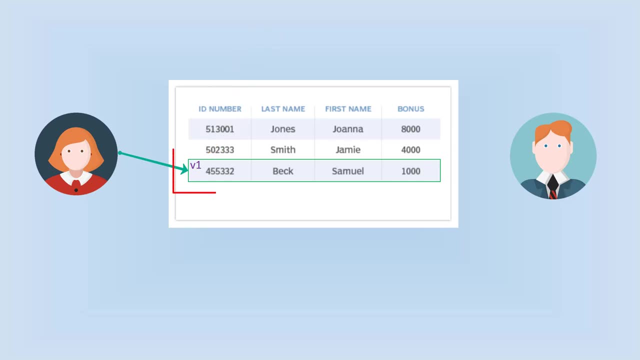 number on the row as well. so every row gets this version number. now, it could be a time stamp, it could be a generated number. how a database does is really up to the database vendor, but let's just say it's a a version number for this case. well, when nick goes in and queries the database and 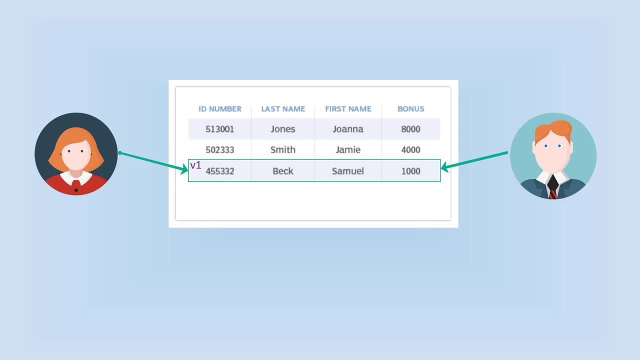 queries. they query it as normal, but part of the query is: give me the highest version number. in this case it's version one. now let's say mike comes in and he wants to write this wrong against samuel beckett. well, what does he do? well, he goes in and he creates a transaction. but instead of 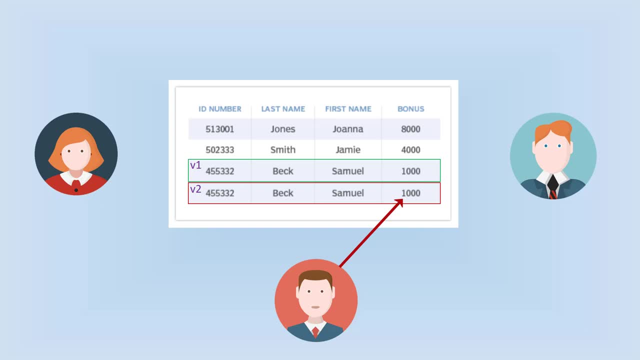 locking that row with multi-version concurrency control, a new row with a new version number is created. now mike does all of his work against that particular row. he updates that row, he works on that row, he edits content in that row and nick and nancy can still query the data because they're. 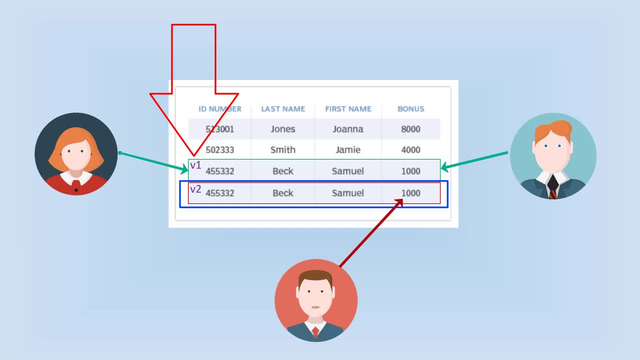 querying version one. right, if nick's transaction hasn't committed, why block out nick and nancy? there's a potential the transaction might fail, in which case the record never gets updated, for that matter. when the record does get updated, well, at that point nick and nancy query that data. so, as you can see here, we're gonna update that record and 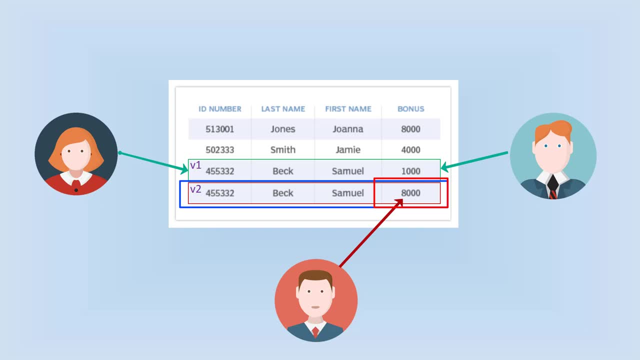 boom. all of a sudden we now see that samuel's bonus is eight thousand. all of a sudden, mike's work is done, so he exits off the stage and what we now have is a new record in this database with a version two number on it. now, the next time nick or nancy or anybody else goes in to. 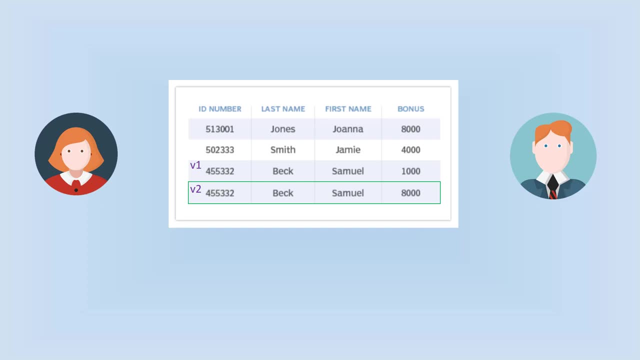 query this database, they'll ask for the record with the highest version number, and what they'll get back is back, samuel beck with the eight thousand dollar bonus, not the one thousand dollar bonus, and so that's the idea of keeping multiple versions of a record in a database. that's the idea of multi-version concurrency control, the idea that you create.